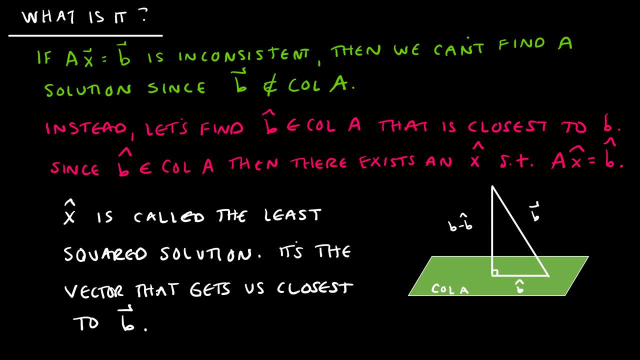 closest to b. So think projections, because that's what we've been working on. So, as we can see in this picture, this parallelogram or plane is the column space of a And b is this vector. Let me change colors. b is my blue vector, Obviously not in the column space of a. 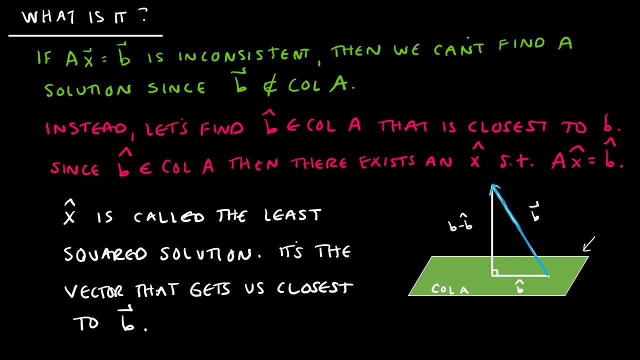 But I can find a projection of that which is right here: b hat Notice. b hat is in the column space of a, So here is b hat in the column space of a, And then of course, this distance or this vector. 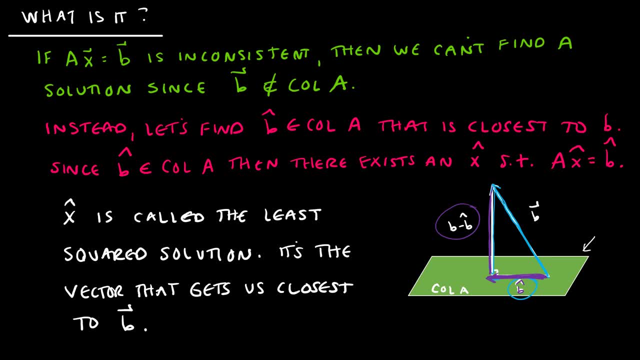 is b minus b hat. b minus b hat is orthogonal to b hat, and it's also orthogonal to every other vector in the column space of a. So what we're saying is we don't have a solution for ax equals b, but we have a solution for ax hat equals b hat and x hat is our least squared solution. 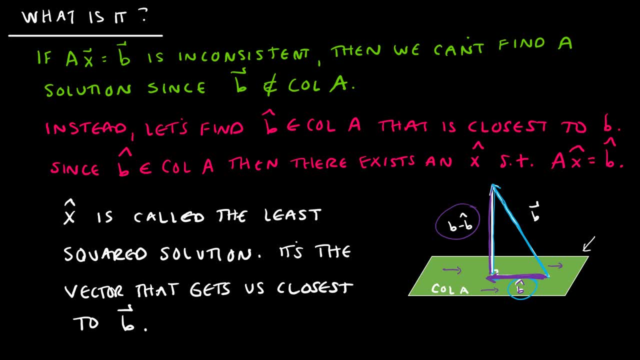 So essentially, it's an estimation. It's an estimation that is the closest. So think about what we've been working on with projections. That's exactly what we're talking about is we're looking at the closest projection. It's the vector that gets us closest to b. 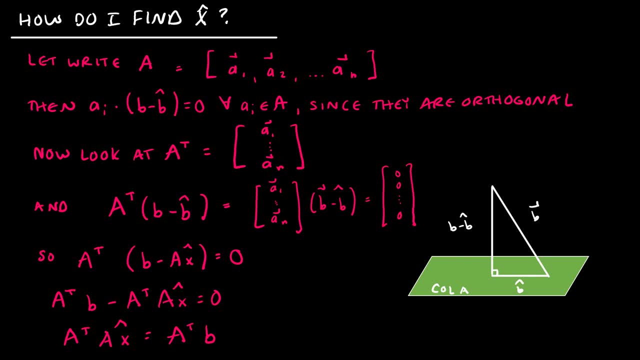 So, knowing that, how am I going to find x hat? So let's think about a. A is just some matrix made of column vectors a1, a2, through an. Then that means if I take each of those column vectors and I dot them with b minus b, 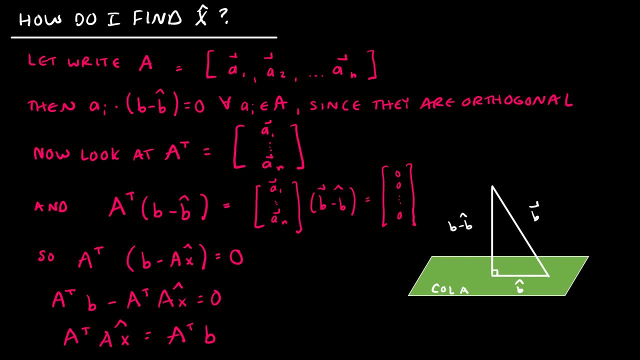 hat, I should get zero. Why is that true? Because we've already said that b minus b hat is orthogonal to the column space of a, because obviously we can see that anything within a is going to be perpendicular to b minus b hat. So everything's orthogonal and therefore 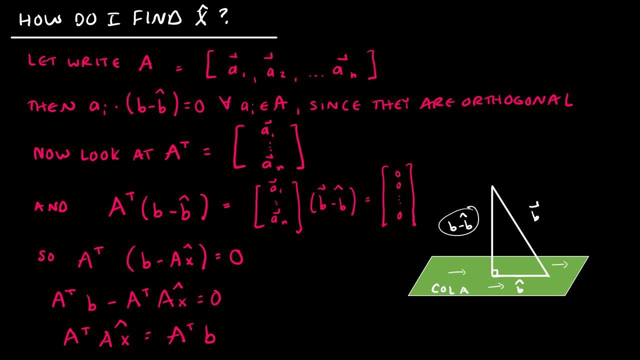 I'm going to get zero. So now, if I look at a and I find the transpose of a, then my columns have now become my rows. And again, if I take transpose and I dot it with b minus b hat, I still get zeros. I get the zero. 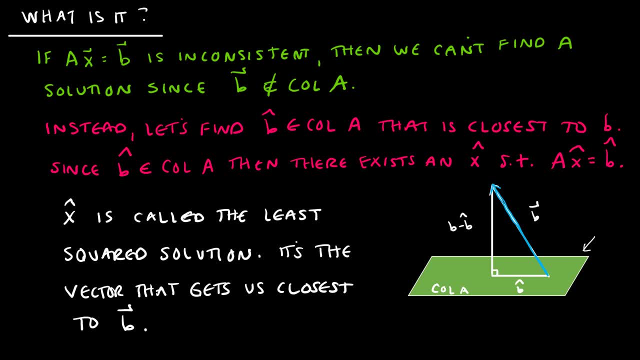 But I can find a projection of that which is right here: B hat Notice. B hat is in the column space of A, So here is B hat in the column space of A, And then of course, this distance or this vector is B minus B hat. B minus B hat is. 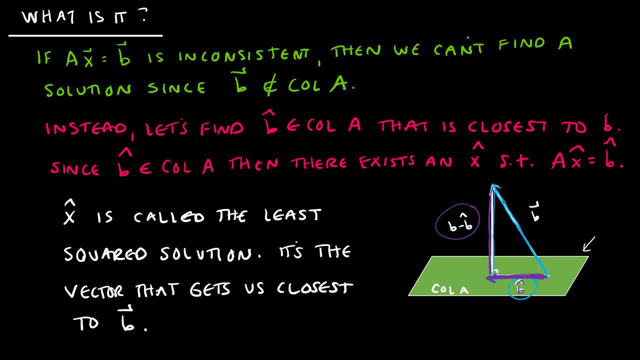 orthogonal to B hat And it's also orthogonal to every other vector in the column space of A. So what we're saying is we don't have a solution for AX equals B, but we have a solution for AX hat equals B hat and X hat is our least squared solution, So essentially it's a. 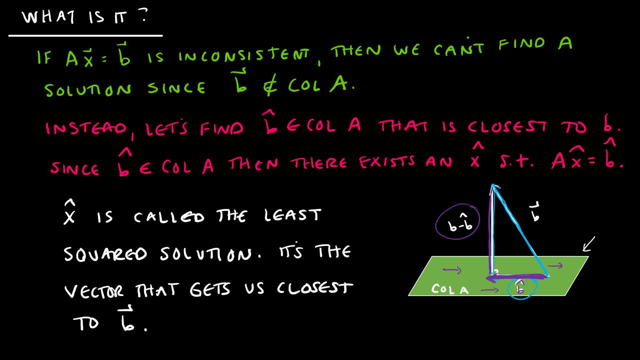 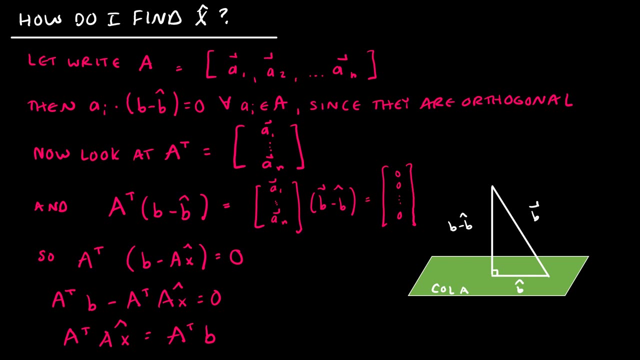 estimation. It's an estimation that is the closest. So think about what we've been working on with projections. That's exactly what we're talking about is we're looking at the closest projection. It's the vector that gets us closest to B. So, knowing that, how am I going to find X hat? 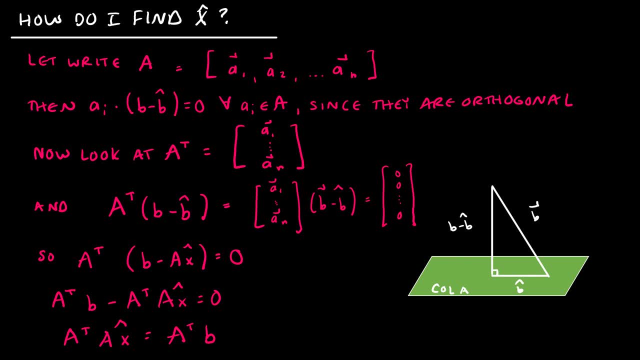 So let's think about A. A is just some matrix made of column vectors A1, A2 through AN. Then that means if I take each of those column vectors and I dot them with B minus B hat, I should get zero. Why is that true? Because we've already said that B minus B hat is orthogonal. 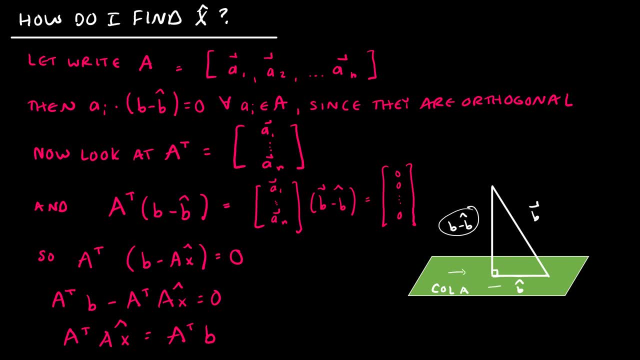 to the column space of A, because obviously we can see that anything within A is going to be perpendicular to B minus B hat. So everything's orthogonal and therefore I'm going to get zero. So now, if I look at A and I find the triangle, I'm going to get zero. So I'm going to get zero. 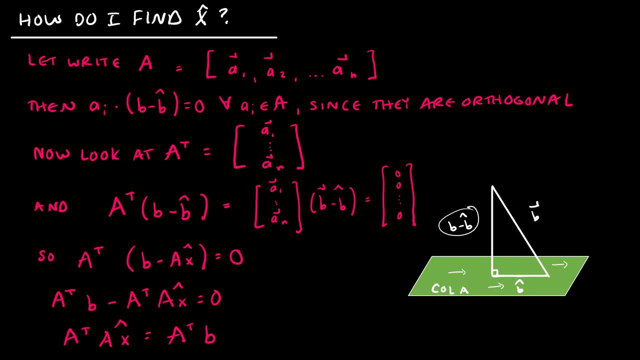 So if I take A transpose of A, then my columns have now become my rows. And again, if I take A transpose and I dot it with B minus B hat, I still get zeros. I get the zero vector. essentially. So that tells me then that A transpose times B minus AX is equal to zero. 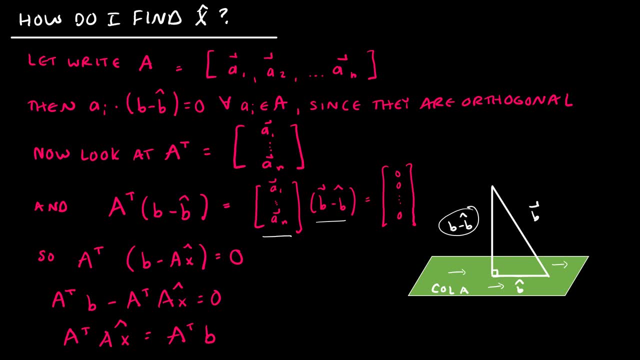 vector essentially. So that tells me then that a transpose times b minus ax is equal to zero. So how did I do that? Well, we talked before about the fact that ax hat is equal to b hat. So this is our estimation. So ax was not equal to b We. 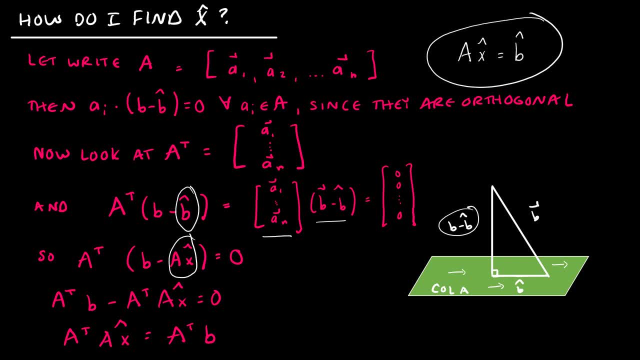 couldn't find a solution. but there is some ax hat that equals b hat. that is our best estimation. So I've just replaced b hat with ax hat and then I've just used some of my properties. So if I have a, transpose times b minus a. 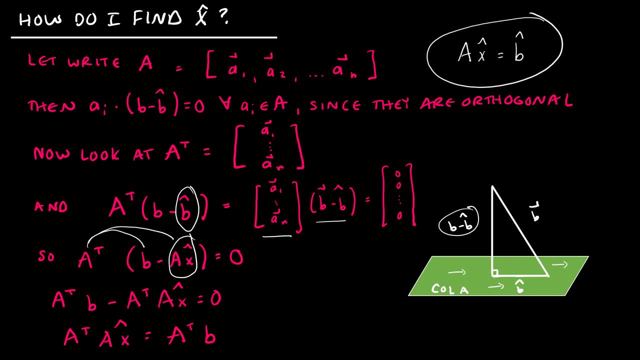 transpose times ax hat equals zero, then I'm just moving this around so that I have these on opposite sides. So I have a transpose ax hat is equal to a transpose b. What is the purpose of all of that? Well, the purpose of all of that- 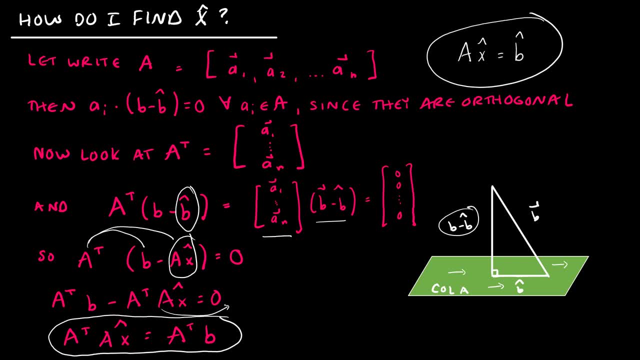 is, I need some strategy or some method in order to be able to help me to find a x hat, because really, what I'm looking for is x hat and this is the only way I can find it. So this is the purpose. We're going to use that to calculate x hat. So let's take a look at an. 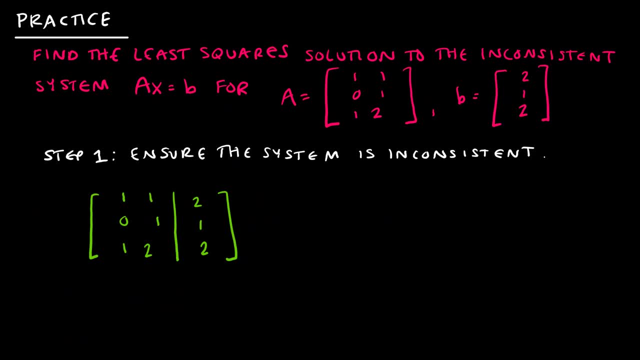 example, The very first thing that I should do is to ensure the system is inconsistent. Now, the way that this question is worded, it says a solution to the inconsistent system. So technically, on this question, I wouldn't necessarily have to check that it's inconsistent, because it makes it pretty clear that it. 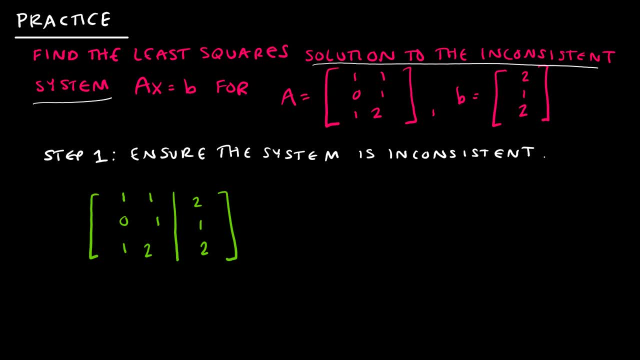 is, but it's not always going to specify that. So let's just remind ourselves how we show that it's inconsistent. So I have my matrix augmented with b, vector b, and all I'm going to do is do some row operations to simplify this a bit. So I'm going to 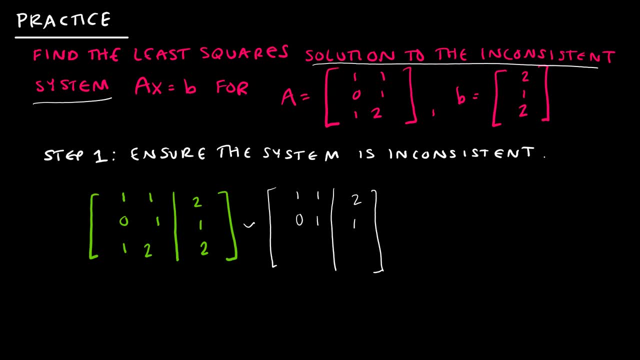 keep my first and second rows the same. My third row. I'm going to take row one minus row three to give me zero negative one, zero. I'm going to continue with my row operations and I'm going to keep my second. first and second row the 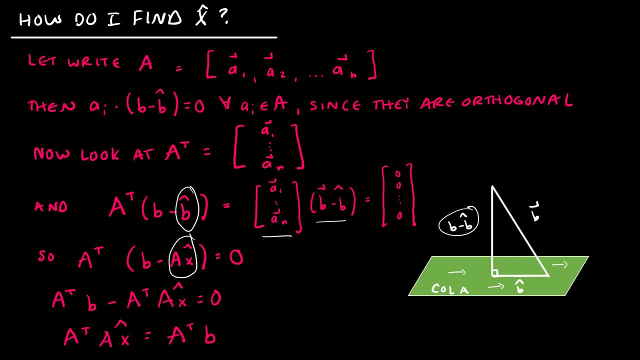 So how did I do that? Well, we talked before about the fact that AX hat is equal to B hat, So this is our estimation. So AX was not equal to B. We couldn't find a solution, but there is some AX hat that equals B hat. that is our best. 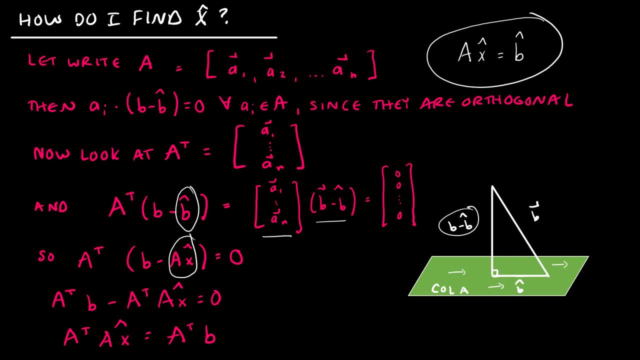 estimation. So I've just replaced B hat with AX hat And then I've just used some of my properties. So if I have A transpose times B minus A transpose times AX hat equals zero, then I'm just moving this around so that I have these on opposite sides. So I have 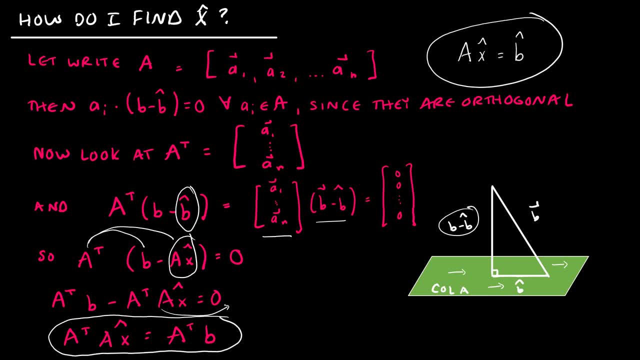 A transpose AX hat is equal to A transpose B. What is the purpose of all of that? Well, the purpose of all of that is I need some strategy or some method in order to be able to help me to find AX hat, because really, what I'm looking for is X hat, and this is the only. 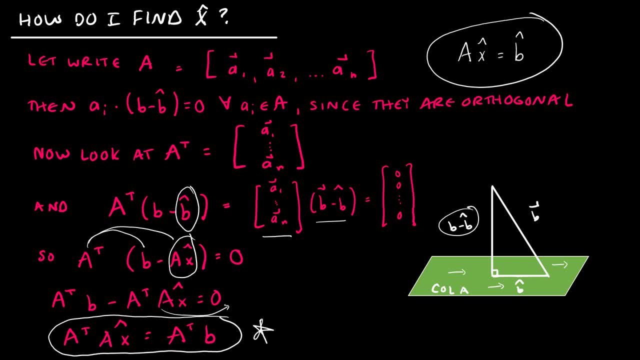 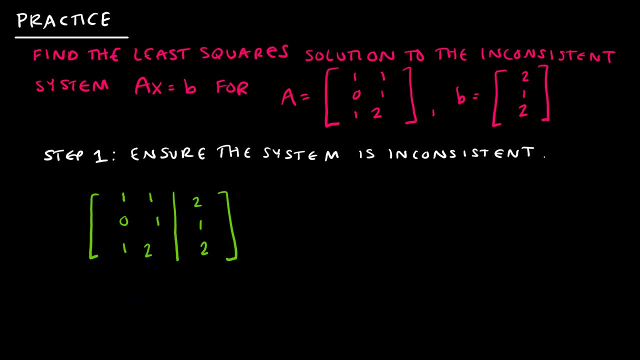 way I can find it. So this is the purpose, That's the goal. We're going to use that to calculate X hat. So let's take a look at an example. The very first thing that I should do is to ensure the system is. 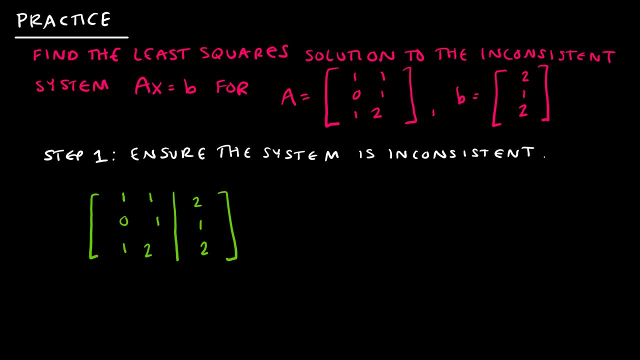 inconsistent. Now the way that this question is worded. it says a solution to the inconsistent system. So technically on this question I wouldn't necessarily have to check that it's inconsistent, because it makes it pretty clear that it is, But it's not always going to specify that. 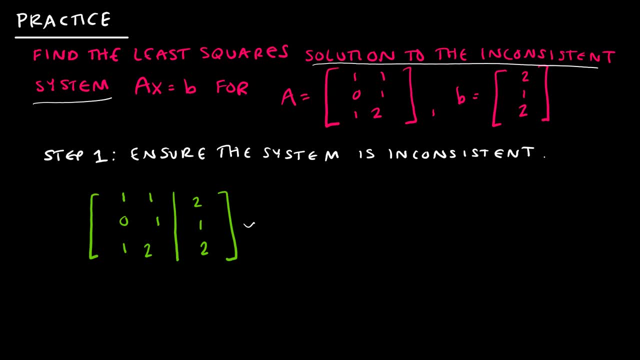 So let's just try to make sure that it's consistent. So let's just try to make sure that it's consistent. So let's just try to make sure that it's consistent. So let's just try to make sure that it's how we show that it's inconsistent. So I have my matrix augmented with B, vector B, and all I'm 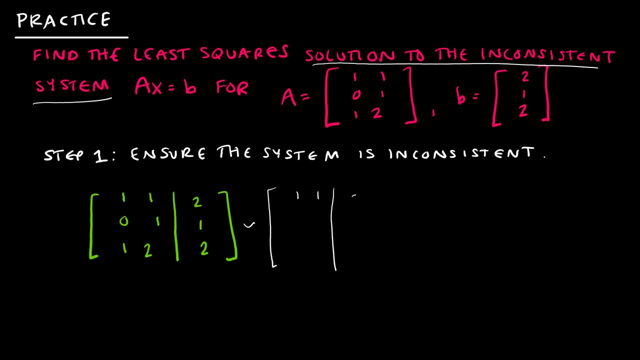 going to do is do some row operations to simplify this a bit. So I'm going to keep my first and second rows the same. My third row, I'm going to take row one minus row three to give me zero negative one, zero. I'm going to continue with my row operations and I'm going to keep my 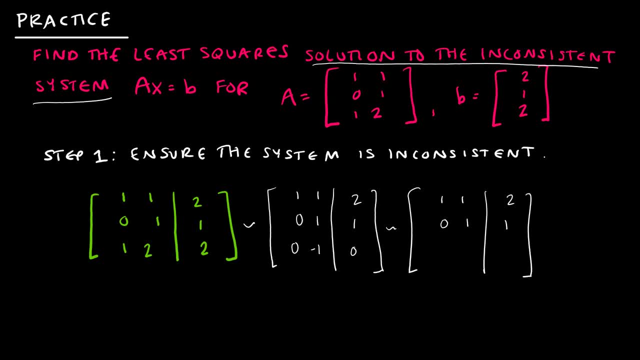 second, first and second row the same, but then I'm going to add rows two and row three together and that gives me 0, 0, 1, and this is how I know that this is an inconsistent system, because this is telling me x1, 0x1 plus 0x2 is equal to 1, and that's impossible, Therefore. 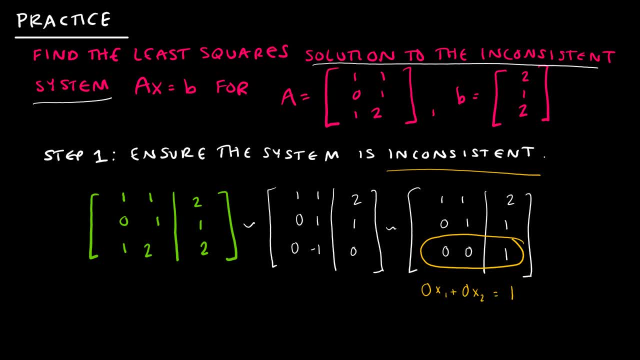 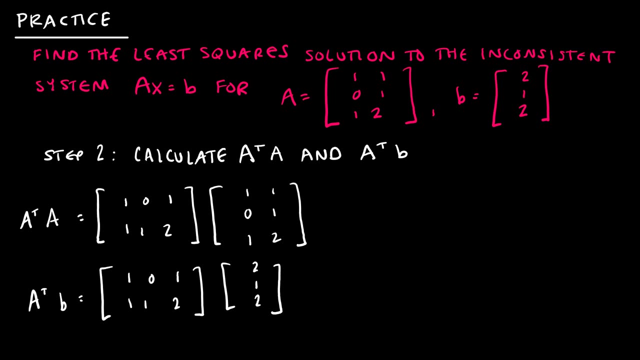 this system is inconsistent and therefore I can't find a solution to ax equals b. However, I can find a least squares solution, so that's what we're going to do. Now that we know for sure the system is inconsistent, let's begin to solve for x. 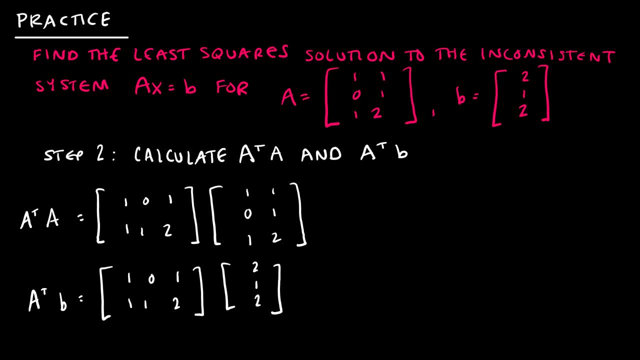 and to begin to solve for x hat. we are looking for a transpose a and a transpose b. So again, I'm just using a, which was given to me, and we know how to find transpose. just turn rows to columns and columns to rows, and I'm going to take that times both. a. 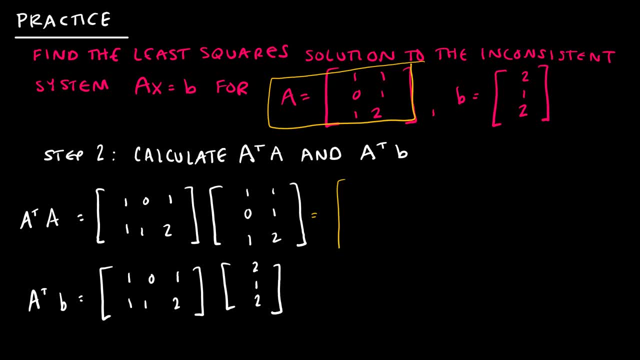 and b, So we all know how to do the math. here I'm going to take 1 times 1,, which is 1, plus 0 times 0,, plus 1 times 1, and then 1 times 1, plus 0 times 1, plus 1 times 2,. 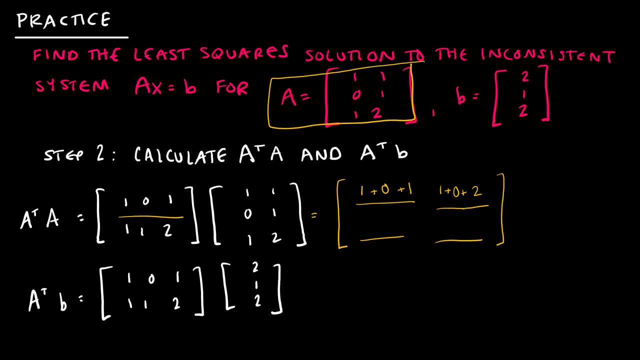 and then, moving on to the next row, I've got 1 times 1, plus 1 times 0, plus 2 times 1, and then 1 times 1, plus 1 times 1, plus 2 times 2,, which means a transpose a. 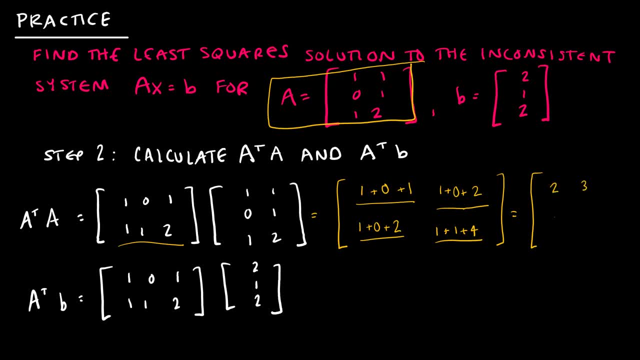 is going to be 2, 3, 3, 6.. I'm going to do the same for a transpose b, so that's going to give me 2 times 1, plus 0 times 1, plus 1 times 2,. 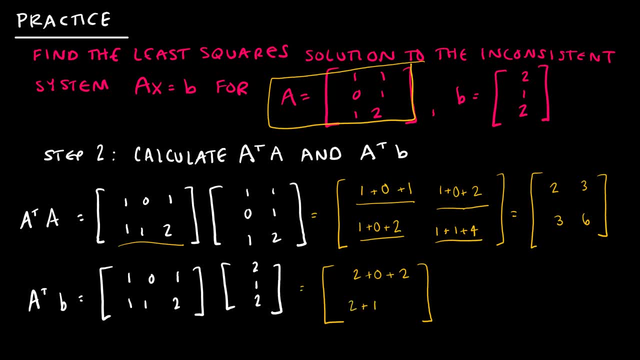 and 1 times 2,, plus 1 times 1, plus 2 times 2, and that gives me 4, 7.. So now I have 2, 3,, 3, 6, and 4, 7, which is a transpose a and a transpose b. And keep in mind my next step. 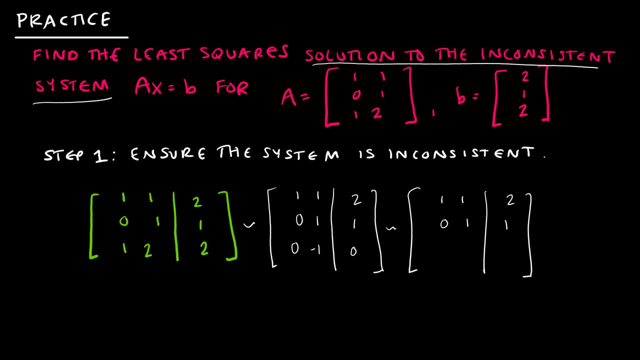 same, but then I'm going to add rows two and row three together and that gives me zero zero one. And this is how I know that this is an inconsistent system, because this is telling me x one, zero x one plus zero x two is equal to one, and 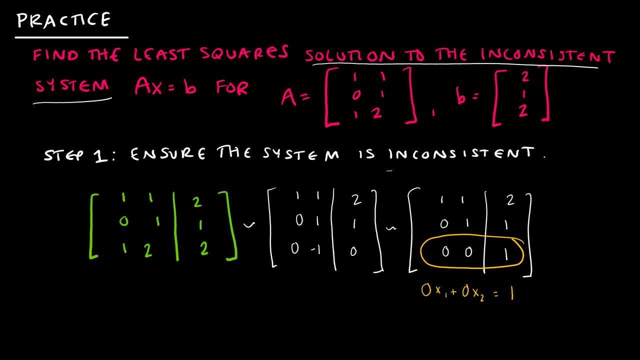 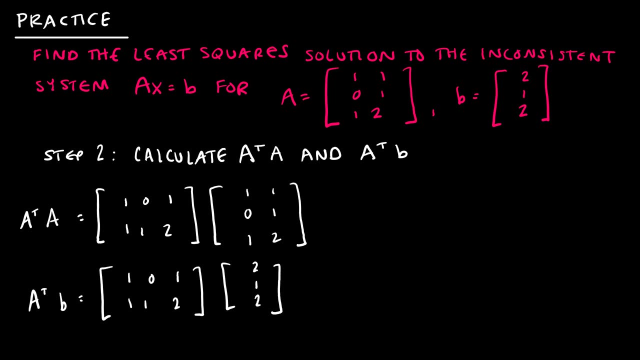 that's impossible. Therefore, this system is inconsistent and therefore I can't find a solution to ax equals b. However, I can find a least squares solution, so that's what we're going to do. Now that we know for sure, the system is inconsistent. 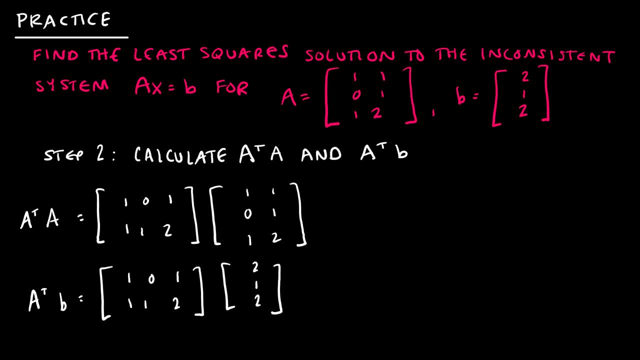 let's begin to solve for x And to begin to solve for x hat we are looking for a transpose a and a transpose b. So again, I'm just using a, which was given to me, and we know how to find transpose: just turn rows to columns and columns to rows. Then I'm going to take 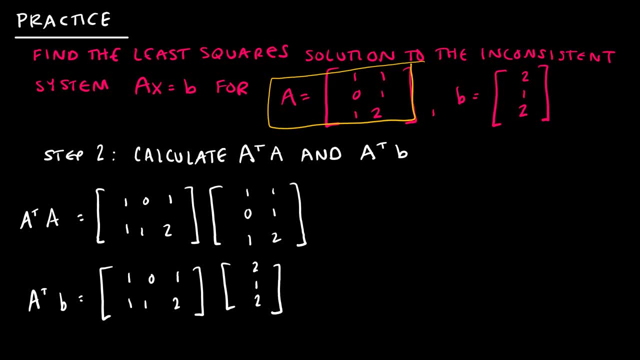 that times both a and b. So we all know how to do the math here. I'm going to take 1 times 1, which is 1 plus 0 times 0 plus 1 times 1, and then 1 times 1 plus 0 times 1 plus 1 times 2.. And then, moving on to the next row, I've got. 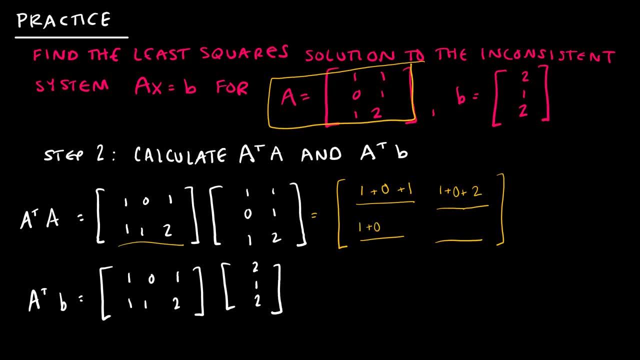 1 times 1 plus 1 times 0 plus 2 times 1, and then 1 times 1 plus 1 times 1 plus 2 times 2, which means A transpose A is going to be 2, 3, 3, 6.. I'm going to do the same for A transpose B. 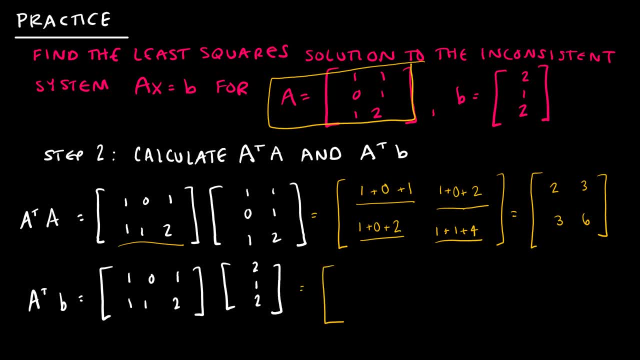 so that's going to give me 2 times 1 plus 0 times 1 plus 1 times 2, and 1 times 2 plus 1 times 1 plus 2 times 2, and that gives me 4,. 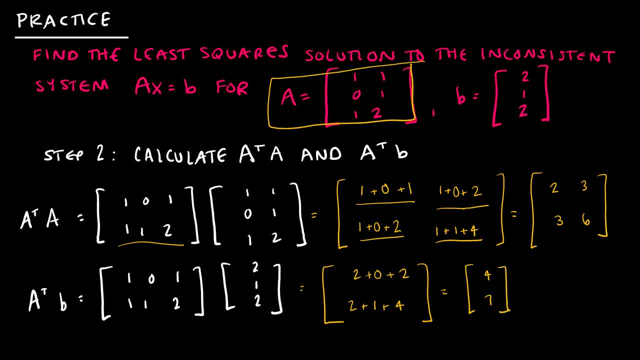 7.. So now I have 2,, 3,, 3,, 6, and 4, 7,, which is A transpose A and A transpose B. and keep in mind: my next step is just going to be using the fact that we learned just a few moments ago that A. 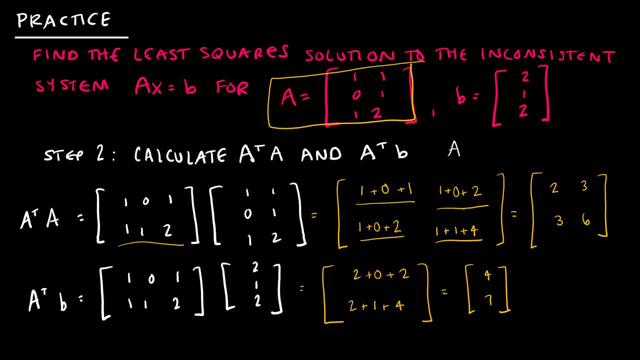 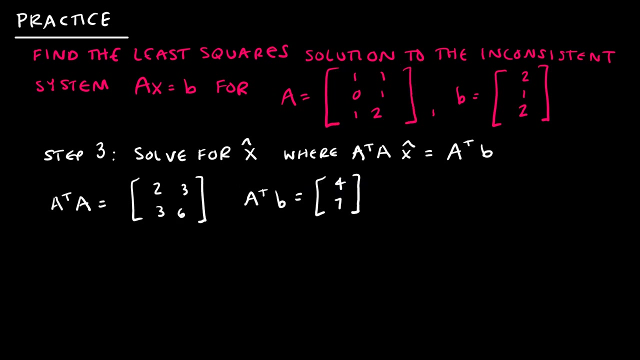 is just going to be using the fact that we learned just a few moments ago that a transpose a x hat is going to be equal to a transpose b. So I have just calculated a transpose a and a transpose b, and all that's left to do is calculate x hat. So how am I going to calculate x hat? Well, 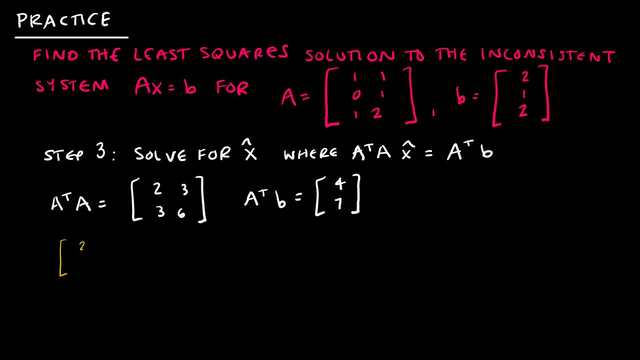 this one's pretty easy. We're back to having our augmented matrix 2, 3, 3, 6, augmented with 4, 7.. So again, I just had to use a transpose a and a transpose b instead. 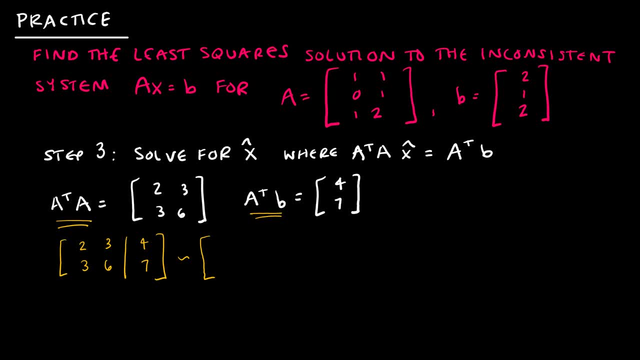 Then I'm just going to do my row operations. So I'll start by taking row 1 times 1 half, So 1, 3 halves 2, and 3, 6, 7.. I'm going to take negative 3 times row 1 and add it to row 2.. So I have 1, 3 halves 2 as row 1,. 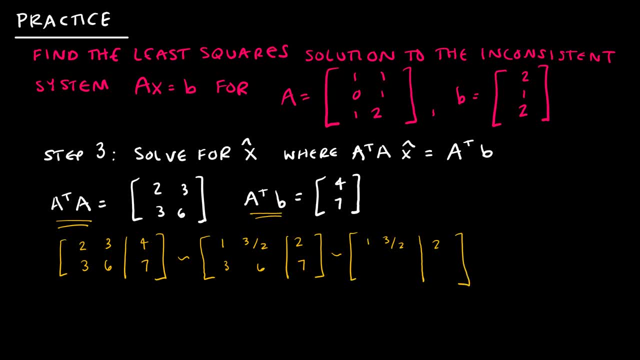 and I'm going to take row 1 times negative 3, which gives me 0,. negative 9 halves plus 12 halves would be 3 halves, and then times 2 times negative, 3 is negative 6, plus 7 is 1.. 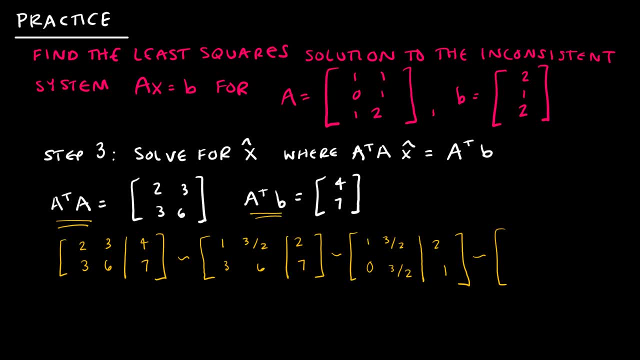 Continuing my row operations, I'm just going to take row 2 and subtract it from row 1.. So that's 1 minus 0, 3 halves minus 3, halves 2 minus 1.. And my second row: I'm just going to take row 2 and subtract it from row 1.. So that's 1 minus 0,, 3 halves minus 3, halves 2 minus 1, and 2.. 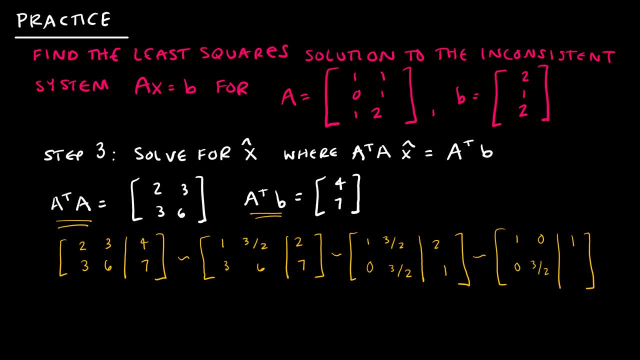 second row is 0, 3 halves 1. I could have done that in another order, but you get the idea, and I've got 1, 0, 1 and I'm going to take that row 2 times 2 thirds. so that's 0, 1, 2 thirds. so what this tells me, then, is that X hat is equal to. 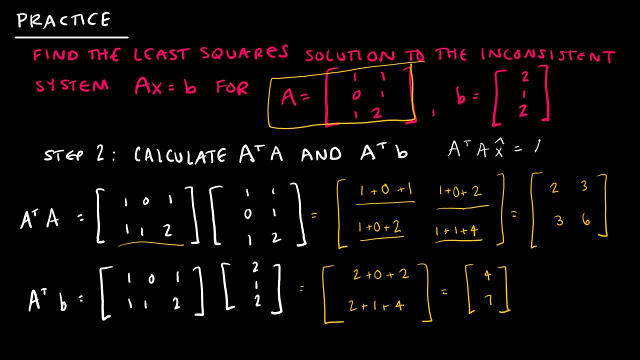 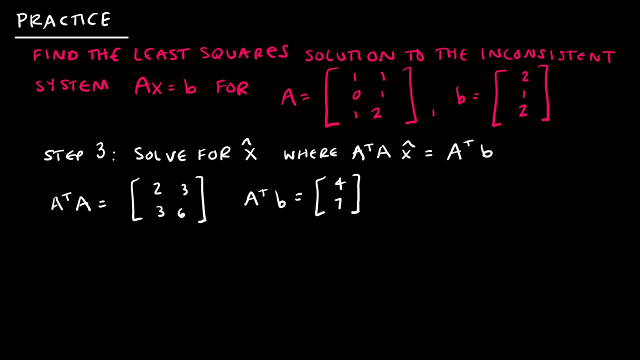 transpose A, X hat is going to be equal to A transpose B. So I have just calculated A transpose A and A transpose B, and all that's left to do is calculate X hat. So how am I going to calculate X hat? Well, this one's pretty easy. We're back to having our augmented matrix: 2,, 3,, 3,, 6,. augmented with 4, 7.. So again, I just have to do a couple of things here. We're going to start with the matrix: 2, 3,, 3, 6,, and then 3,, 3,, 3, 6, augmented with 4, 7.. So again, I just have to do a couple of things here. We're going to 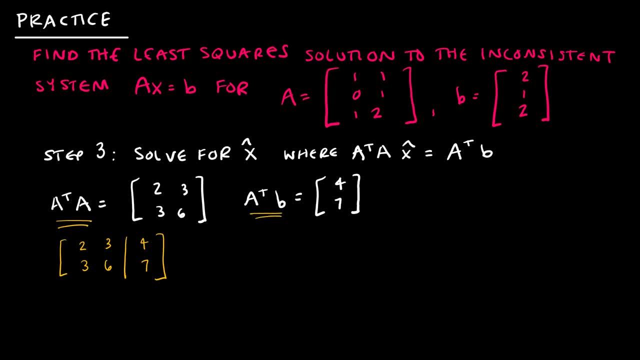 to use A transpose A and A transpose B instead, and I'm just going to do my row operations. So I'll start by taking row 1 times 1 half, so 1, 3 halves 2, and 3, 6, 7.. I'm going to take 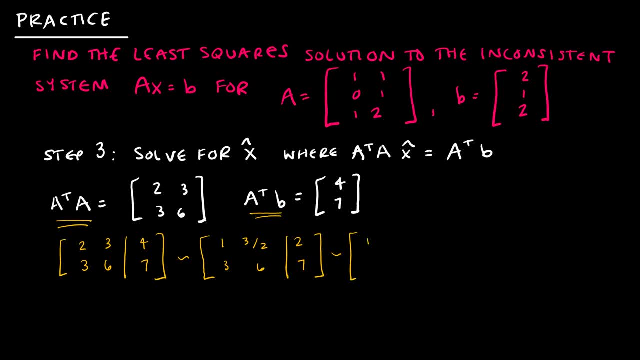 negative 3 times row 1 and add it to row 2, so I have 1,, 3 halves, 2 as row 1, and I'm going to take row 1 times negative 3, which gives me 0, negative 9 halves plus 12 halves would be 3 halves. 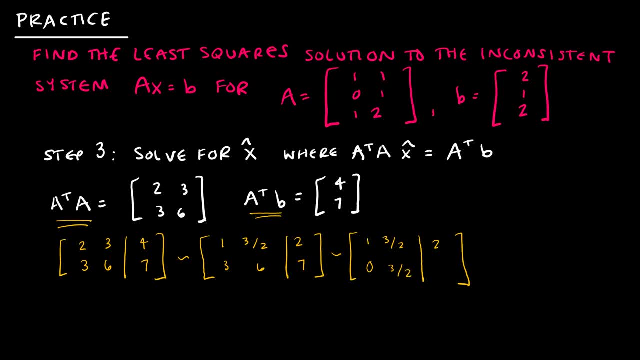 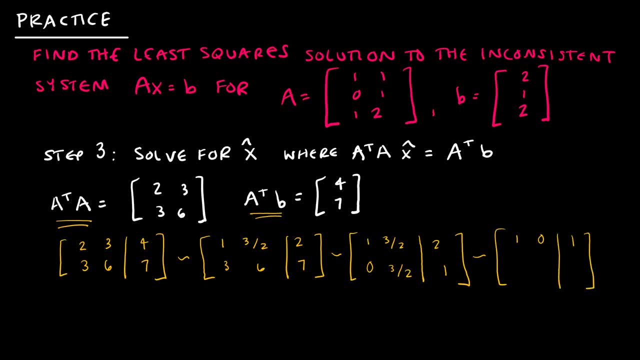 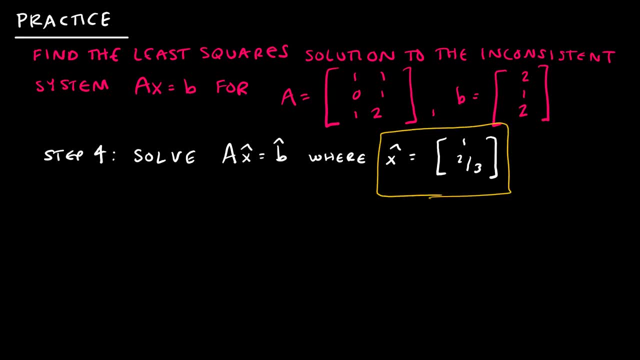 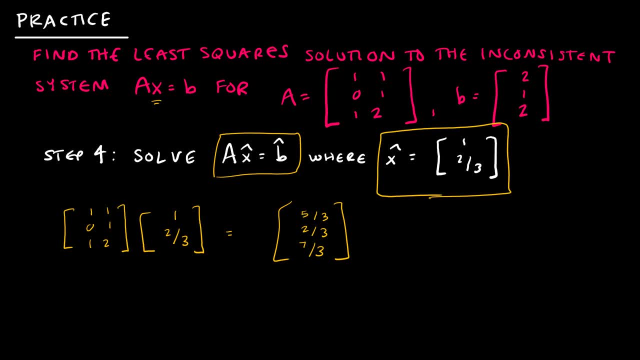 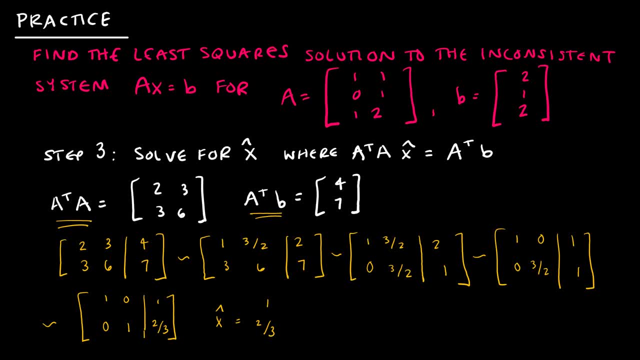 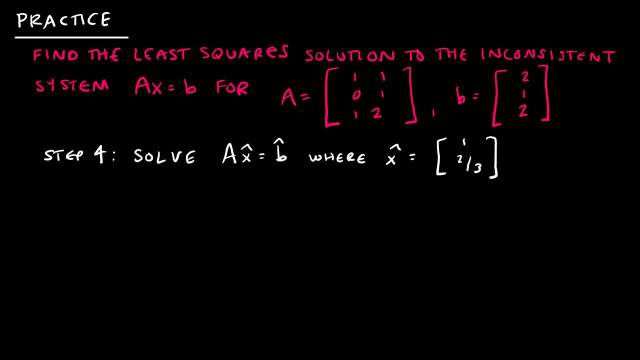 1, 2 thirds. so now I know X hat is 1, 2 thirds, but I'm still not done, because my question said: solve the system for the least squares solution and I still haven't done that because I haven't found B hat, I found X hat, so that's really good. 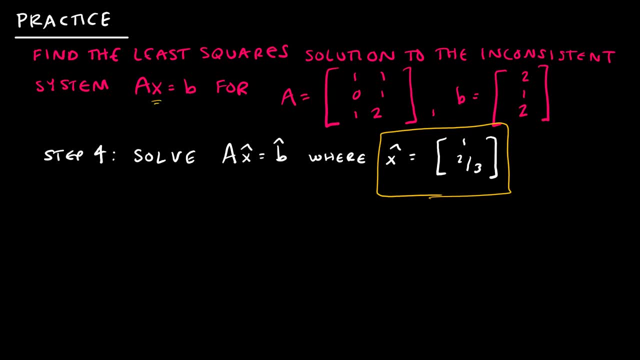 because that is my estimation of X, X and B is not a solution. so essentially I need to continue now to find B hat, because we remember that a X hat is equal to B hat. so now I'm going to take a, which is 1: 1 0, 1, 1, 2. I'm going to take it times the X hat that I just found in. 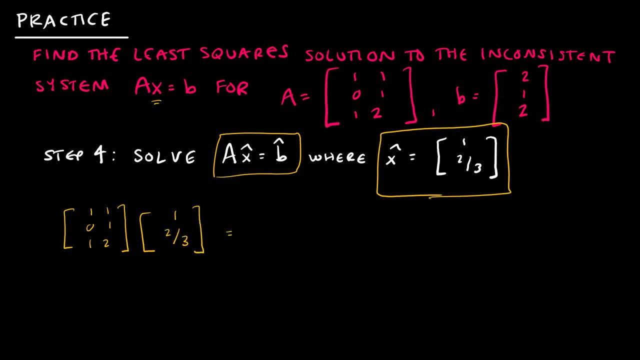 my last step: 1, 2 thirds and that's going to give me B hat, which is my estimate to my vector B. so that's going to give me 1 plus 2 thirds, which is 5 thirds. that's going to give me 0 plus 2 thirds, which is 2 thirds, and 1 plus. 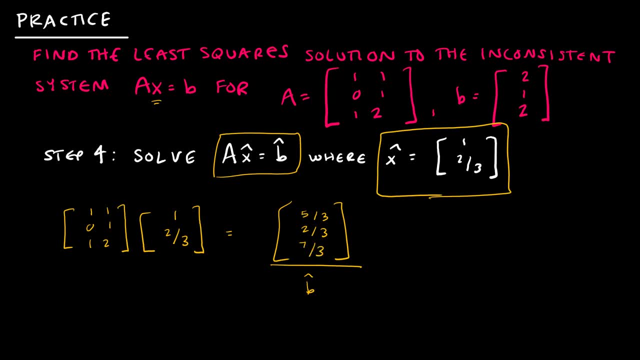 four-thirds, which is 7 thirds. so what have I found? I know that X hat is 1, 2 thirds. I know that b is five thirds, two thirds, seven thirds. So now let's think about what this means. Remember that our goal was to solve for x hat, which we did, and then we need to know. 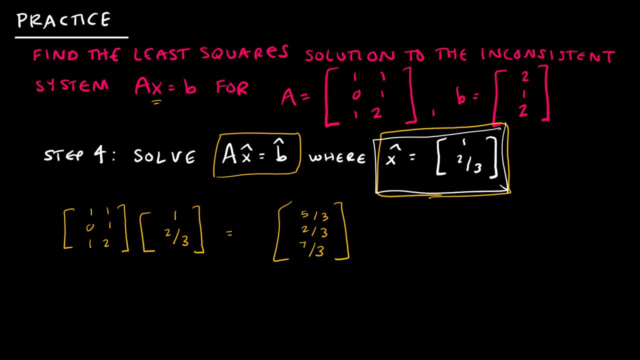 what kind of error are we dealing with? So if it just said solve, I could have stopped at step three, because I found that x hat was one, two thirds, which is my estimate for x. that I would multiply by a to get my estimate for b. But typically we also want to know what we're dealing with. 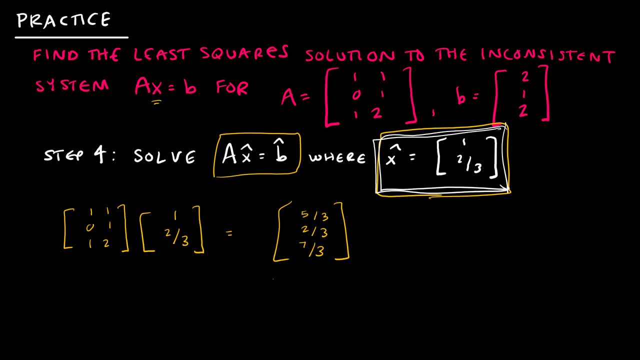 in terms of error. So this again is b hat, It's my estimate for b And I want you to compare that to my actual b, which was two, one, two. Five thirds is just a little bit less than two, Two thirds is a little bit less than one and seven thirds is a little bit more. 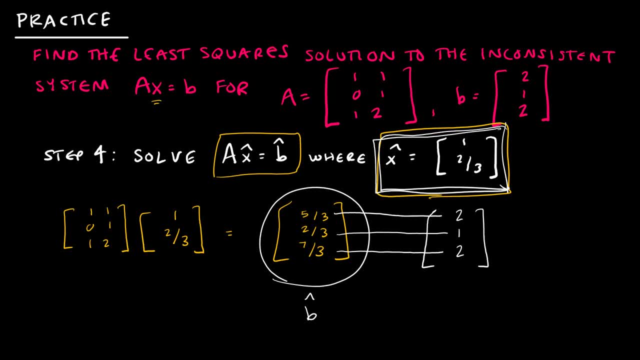 than two. So we can see that b hat is an estimation or a close approximation of b. So I feel pretty good about our solution. but typically from here they could ask us to then talk about the error. So the error is, instead of just comparing b hat and b and saying, hey, 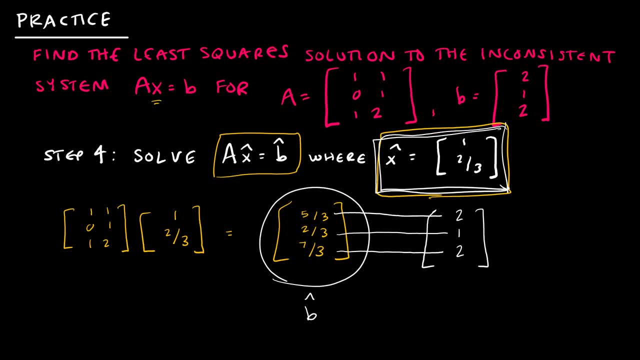 look, they're really close. We're going to say how close are they? So, to answer the how close are they question, I'm just going to say how close are they And then I'm going to say how close are they. And then I'm going to say how close are they And then I'm just going to 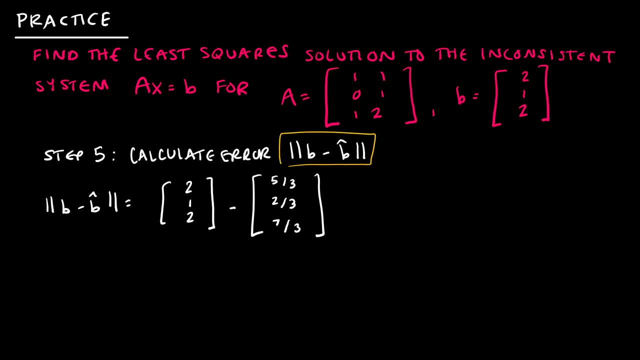 find the magnitude of b minus b hat. So I'm going to take b minus b hat, which is two minus five thirds, which is one third, And one minus two thirds, which is one third, And two minus seven thirds, which is negative one third, And I want to find the magnitude of that And if you'll recall, 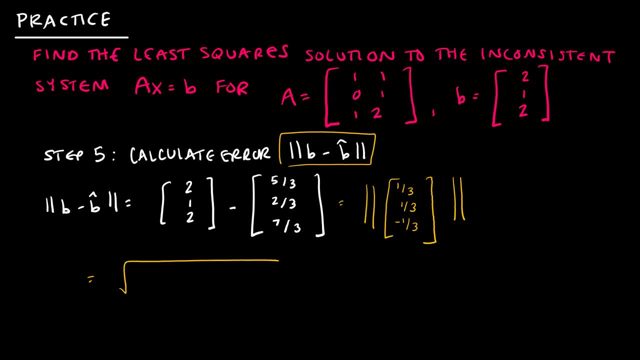 the magnitude of that is the square root of each of those, the each of those values squared. So one third squared plus one third squared plus negative one third squared, which gives me the square root of one third or one third root three. This is my error, that's my magnitude. So if they talk about how large the error is. that's what we're going to do. So I'm going to say how close are they? And then I'm going to say how close are they. So if they talk about how large the error is, that's my magnitude. 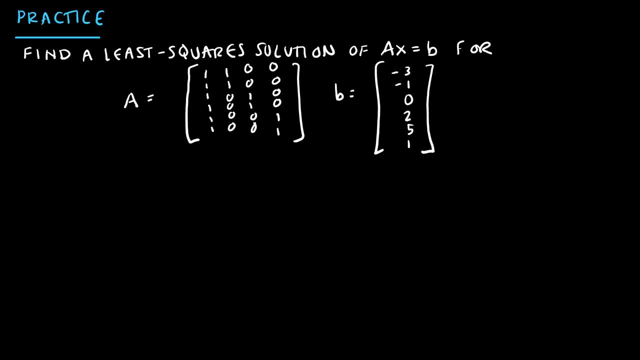 And, if you'll recall, I said b is thejsk and b minus b. hat in theły is squared. I definitely didn't şu Yet Because I didn't realize we were neat, But we did. Yep, okay, not so good. 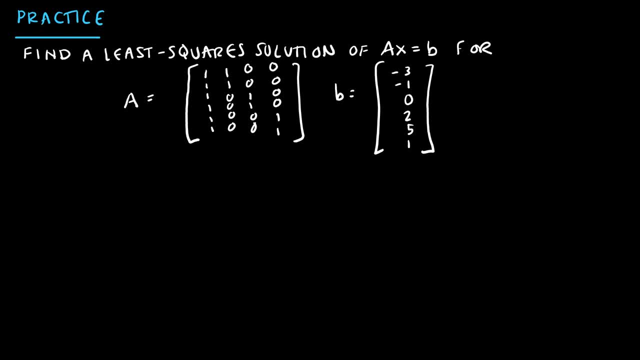 thing we would do is discover that it is, in fact, an inconsistent system, and I'm just going to say that I checked that Inconsistent check, check. So I trust that you have done that, that you checked to make sure that I ended up with a solution that didn't work out, for AX equals B, Step two: 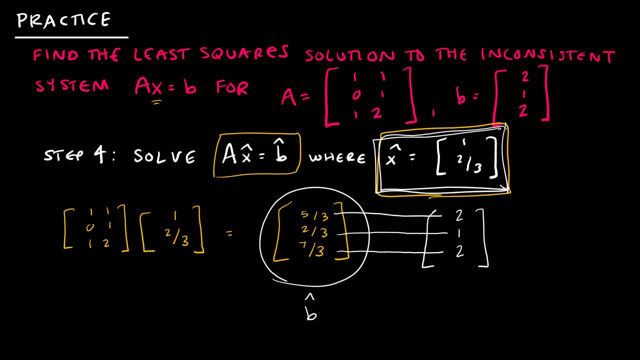 or a close approximation of b. So I feel pretty good about our solution. but typically from here they could ask us to then talk about the error. So the error is, instead of just comparing b, hat and b and saying, hey look, they're really close, we're going to say how close are they? 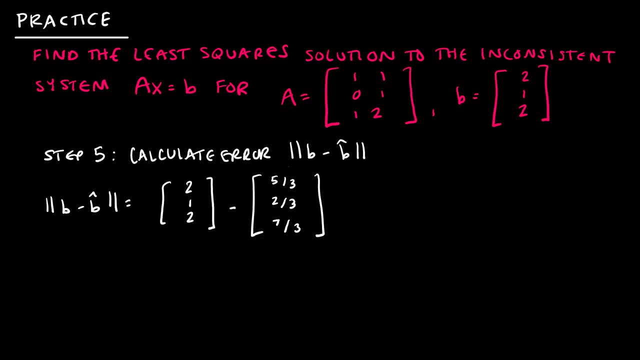 So to answer the how close are they question, I'm just going to find the magnitude of b minus b hat. so I'm going to take b minus b hat, which is 2 minus 5 thirds, which is 1 third, and 1 minus 2 thirds, which is 1 third, and 2 minus 7 thirds, which is negative 1 third, and I want to 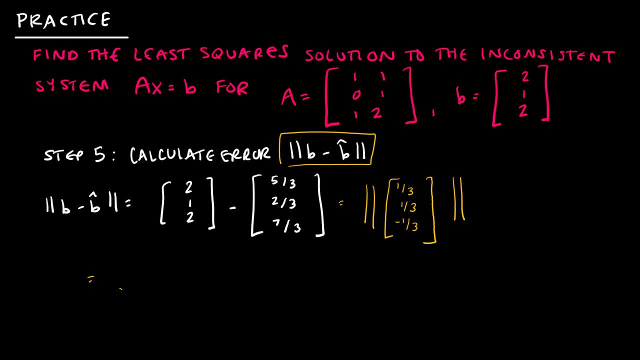 find the magnitude of that and, if you'll recall, the magnitude of that is the square root of each of those, the each of those values squared. So 1 third squared plus 1 third squared plus negative 1 third squared, which gives me the square root of 1 third or 1 third root 3.. This is my error, that's my magnitude. 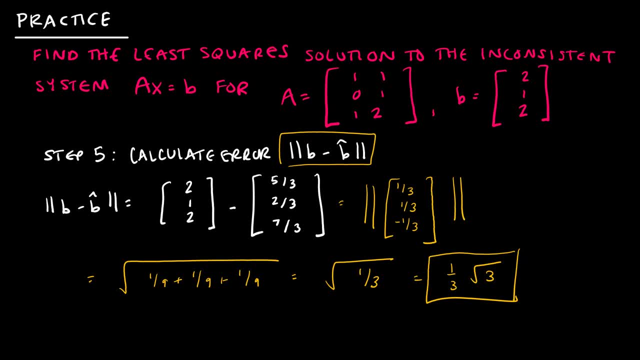 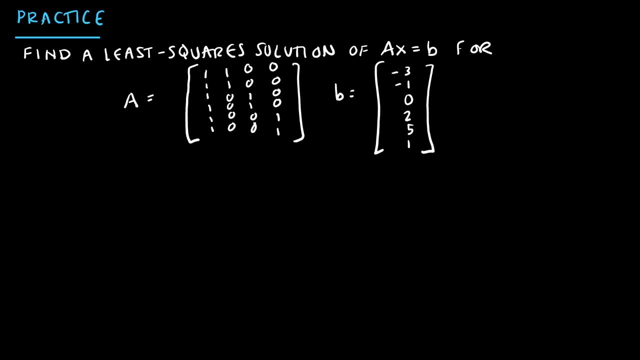 so if they talk about how large the error is, that's what we're looking at- is the magnitude. Here's one question for you to try for us to finish up- and again, I'm not going to show all of the work when we go through this solution together, but just know that when you do this one, you should end up. 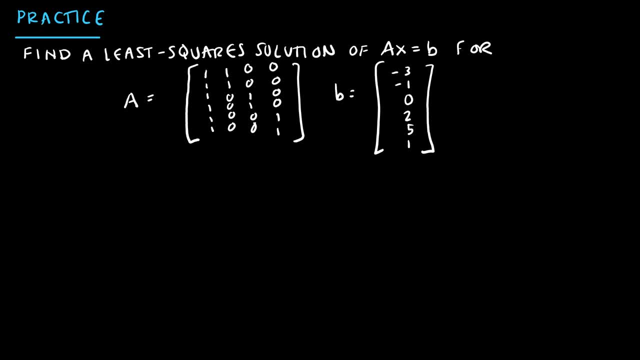 with a free variable or two. so your solution is going to look a little bit different than the last question. So do press pause. try this question. it might take you a couple of minutes and that's okay. when you're ready, press play to see how you did. So remember, first thing we would do is discover: 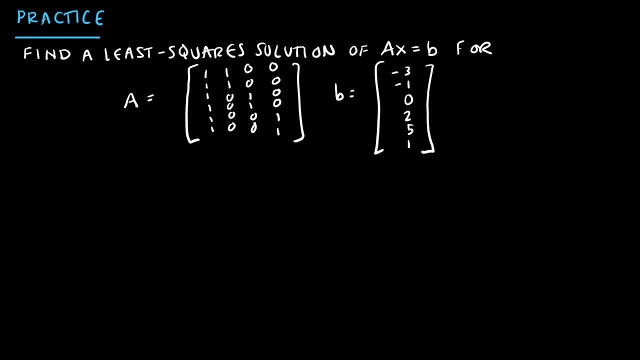 which one of these twoệthe in the- This is in part, what stain is half of What the formula is for this. Let's say I did not find this value here. What do I do? Well, have enough room on this slide to show everything, But you should have gotten 6222,, 2200,, 2020, 2002.. 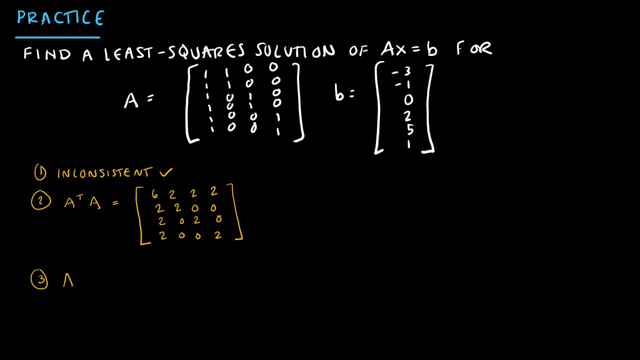 Step three is to find A, transpose B And again, I'm not going to show the work, but you should have ended up with 4, negative 4, 2, 6.. Step four is to write it as an augmented matrix, which means I'm going to write 6222, 4, 2200, negative 4, 20202, and 2002, 6.. 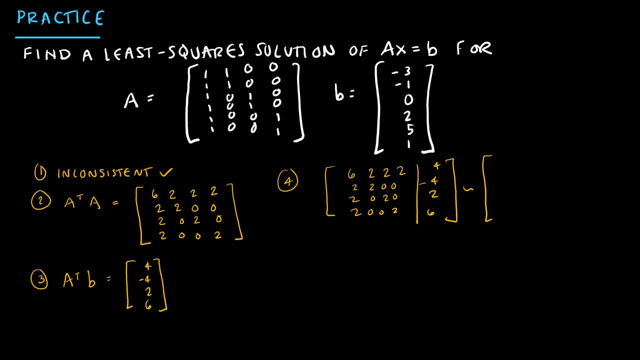 And magic With a row reduction calculator, I would end up with 10013, and 010,, negative 15, and 001,, negative 1,, negative 2, and 00000.. So, yay, free variables. Which means now, and this one I didn't have to do on my last example, but now I'm going. 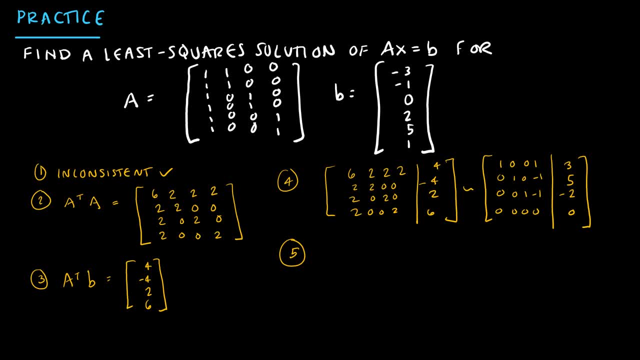 to have to write it as a row reduction calculator. So I'm going to write the general solution And the general solution we know how to do, because obviously this first row just says: x1 plus x4 is equal to 3, etc. 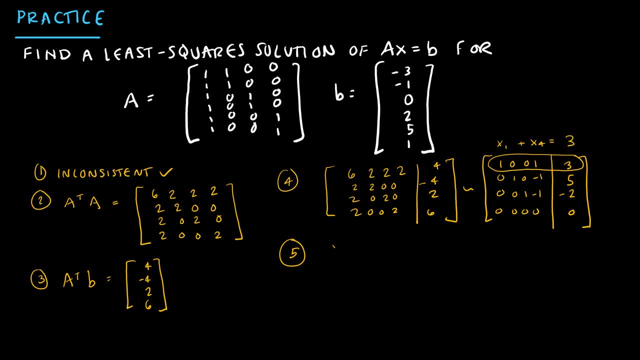 And so what I would write is that x1 is equal to 3 minus x4,, that x2 is equal to 5 plus x4,, that x3. is equal to negative 2 plus x4,, which means my solution, which is x1, x2, x3, x4, can. 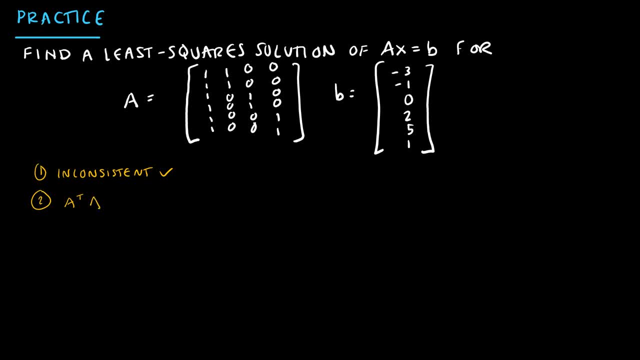 remember is to find A transpose times A, and I'm not going to show those calculations just because I don't have enough room on this slide to show everything, but you should have gotten 6222,, 2200, 2020, 2002.. Step three is to find A transpose B and again. 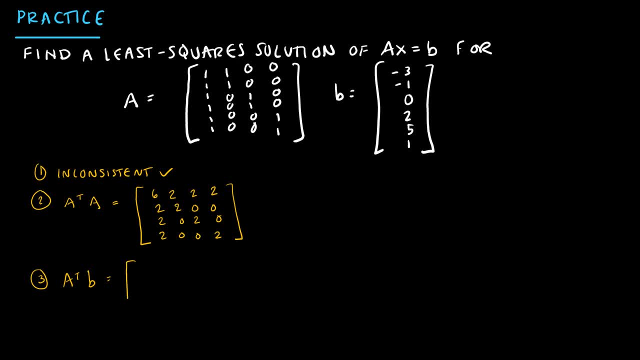 I'm not going to show the work, but you should have ended up with 4, negative 4, 2, 6.. Step four is to write it as an augmented matrix, which means I'm going to write 6222,, 4,, 2200, negative 4, 20202, and 2002, 6,. 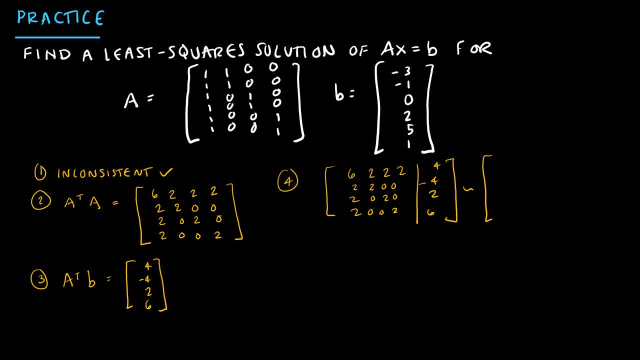 and magically, with a row reduction calculator, I would end up with 10013, and 0, 1, 0, negative 1, 5, and 0, 0, 1, negative 1, negative 2, and 0, 0, 0, 0, 0.. So, yay, free variables, which means now: 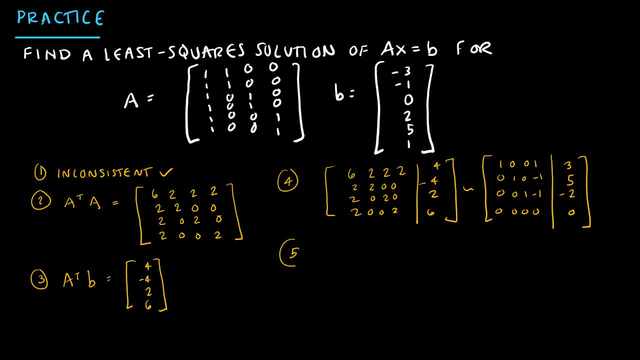 and this one I didn't have to do on my last example, but now I'm going to have to write the general solution, and the general solution we know how to do, because obviously this first row just says: X1 plus X4 is equal to 3, etc. 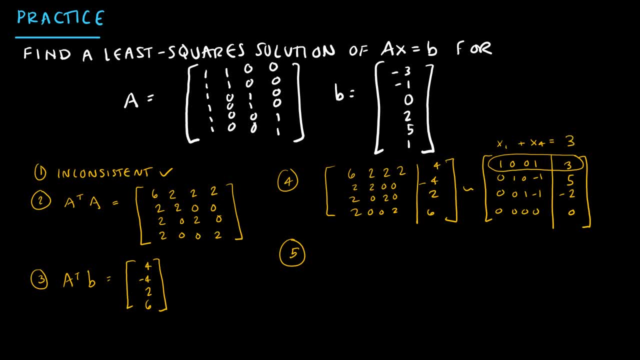 and so what I would write is that X1 is equal to 3 minus X4,, that X2 is equal to 5 plus X4, X3 is equal to negative 2 plus X4, which means my solution, which is X1, X2, X3, X4, can.